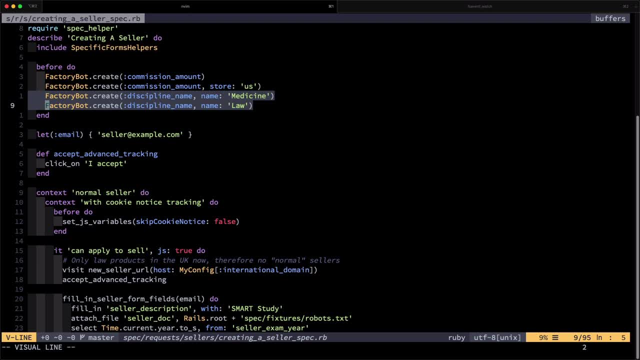 selling in order to populate the form where the seller chooses what they're going to sell. So I'm going to populate the form where the seller chooses what discipline they'd like to sell on the website. There's also this email which the prospective seller is going to type into that. 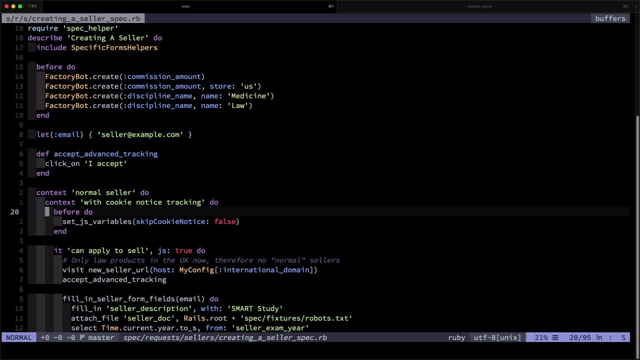 form. I share this throughout all the examples here. Now let's skip down to the test itself. It's JS, true? This essentially means that we're going to use a JavaScript driver as opposed to a purely HTML driver. What actually happens in the test? We visit some particular URL. 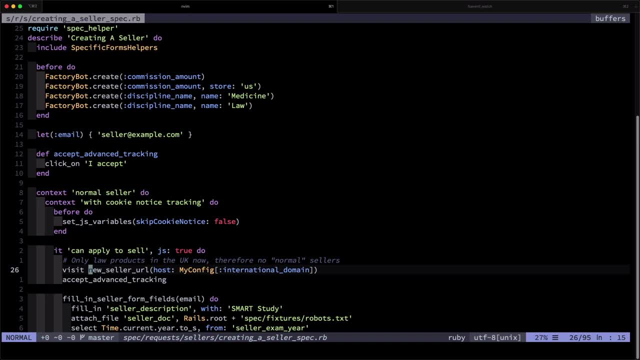 the new seller URL. This is a named URL which turns into the actual URL. We accept some advanced tracking. This is defined over here. It just means click on I accept in the JavaScript thing. Then we fill in seller form fields. This is also a custom piece. 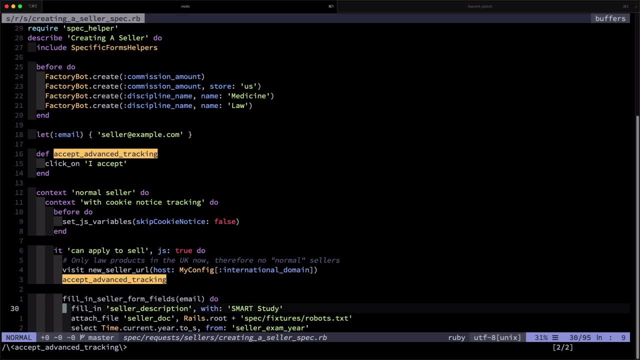 of code because I share this throughout multiple tests and it gets modified here with some extra fields. I fill in seller description with the text smart study. I attach a file to the seller doc ID and that file is found in railsroot plus some particular fixtures, the robotstxt. I use that. 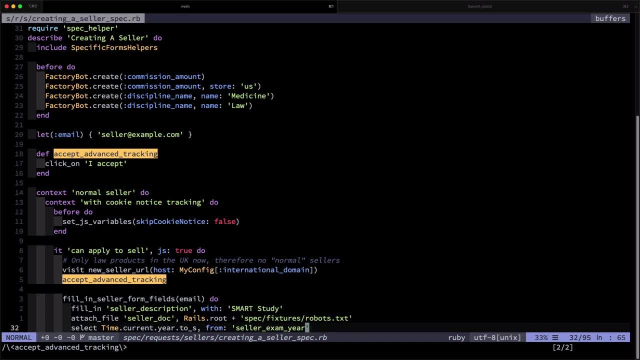 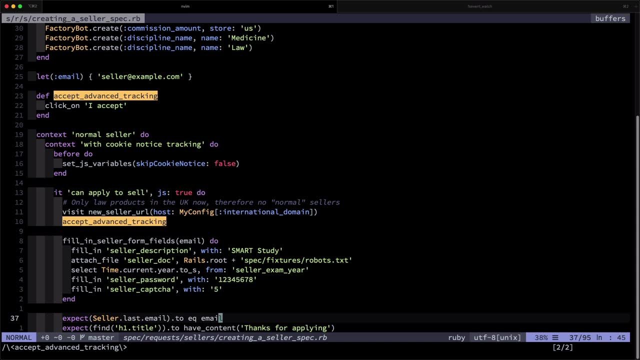 particular file because it's extremely small and the test will run more quickly. I select the current year from seller exam year And so I'm going to use the current year from seller exam year on and so forth. Once all that's done, I start running my sort of test assertions to check that. 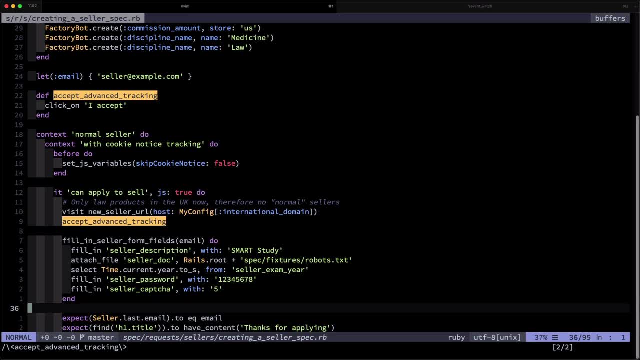 everything worked. The first thing, the main thing I expect is that a seller has been created in the database And I check here that the last seller's email is equal to the email which I provided up above seller at examplecom. Then I check that the h1.title on the final page has the content: 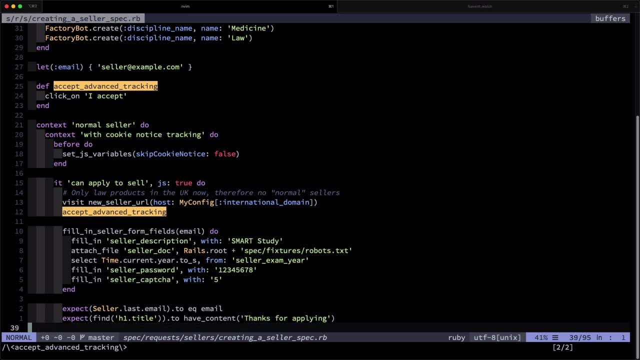 thanks for applying ie that the seller gets moved on to the next page And then I do some sort of JavaScript testing. I check that the h1.title on the final page has the content thanks for applying. ie that the seller gets moved on to the next page And then I do some sort of JavaScript testing. I. 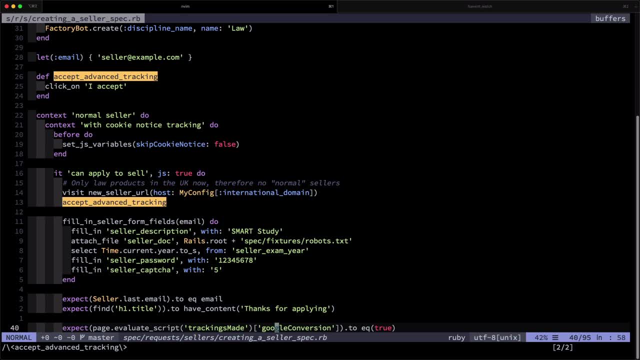 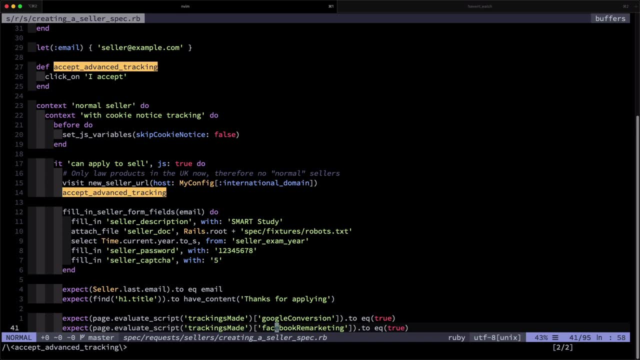 evaluate some custom JavaScript and I check that the trackings made object has Google conversion- true. What I'm essentially doing here is checking that my tracking code works. I find this is very fragile, so therefore I test this in my integration tests. All of this is really nice. I find it reads: 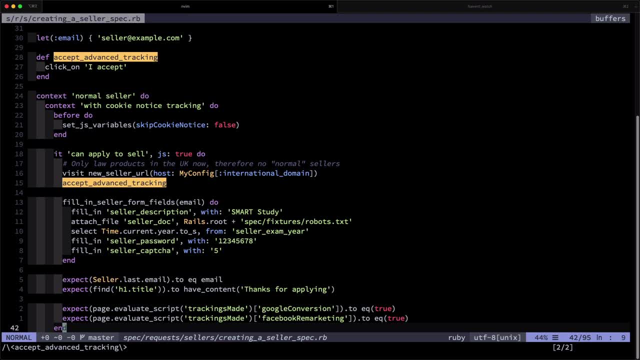 almost like English, especially this stuff for visiting URLs, filling in form fields, attaching files. It's one of the easiest things you can possibly code and it takes very little time to do it, once you've learned the basic syntax. And don't be fooled into thinking that this is a 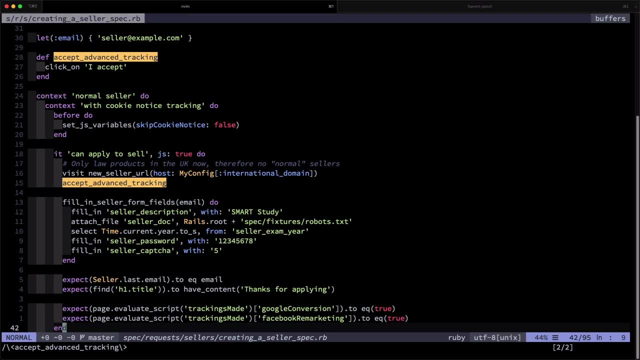 Ruby or Rails specific thing. I've used almost the equivalent library in PHP Laravel. it's called Dusk, and there's something very similar in JavaScript and Python too. I believe this exists in every programming language out there. Before I had these tests in place, working with my codebase. 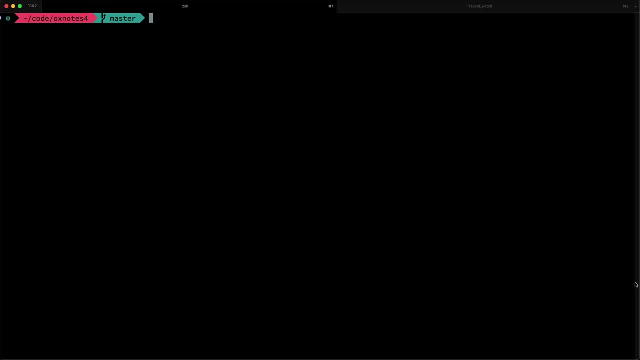 was a bit like whack-a-mole: I'd change some feature and then randomly, or seemingly randomly, in some far away part of the code something would break, and I'd find out about that two days later and then be up in the middle of the night trying to fix it. Then one winter, 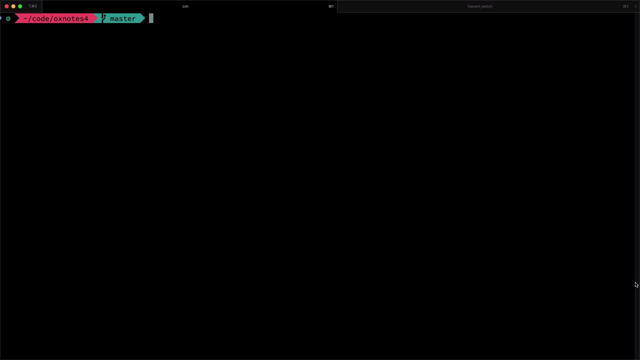 about five or six years ago when I was in Rio. at the time, I spent every single morning adding tests to my existing codebase. Let's see how many of them I added in total using ripgrep. So I'm going to ripgrep for the start of a line and then a space or multiple spaces. 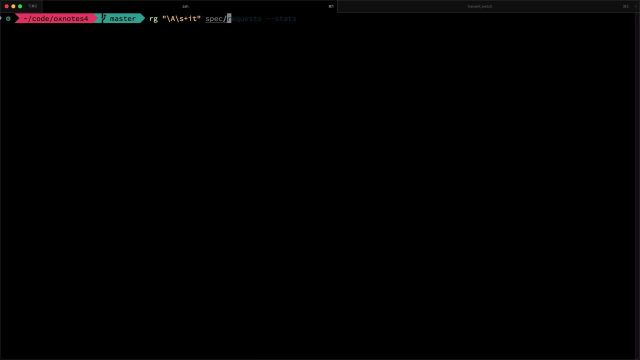 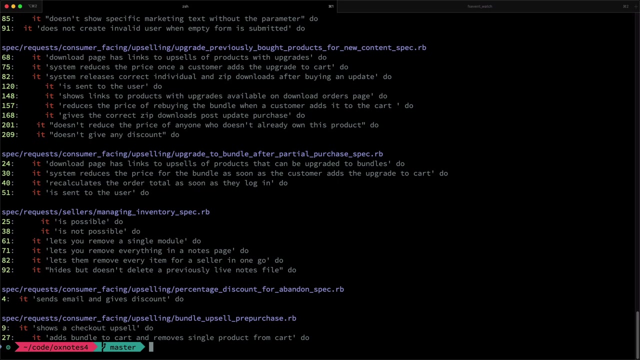 possibly, I don't care how many. Then the word it and I'm just going to run that little search within spec requests. That looks about right. You can see that all these tests are occurring. For example, it shows a checkout upsell, It adds bundle to cart and removes single product from. 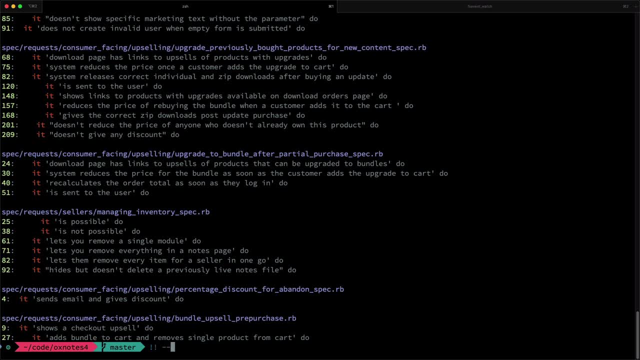 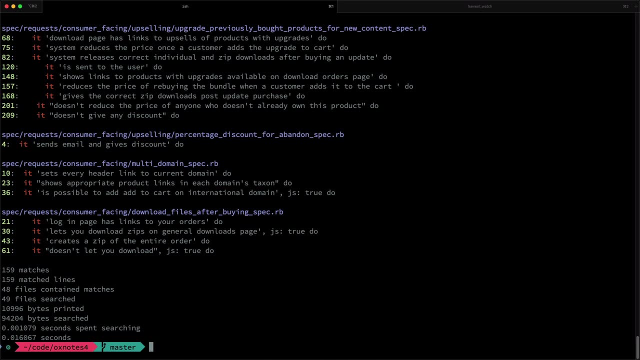 cart. Now let's see how many of them I have in total. I'm going to rerun that command with the stats flag and you can see there that I have 159 matches, 159 of these integration tests. I love having these. Now that I have them in place. 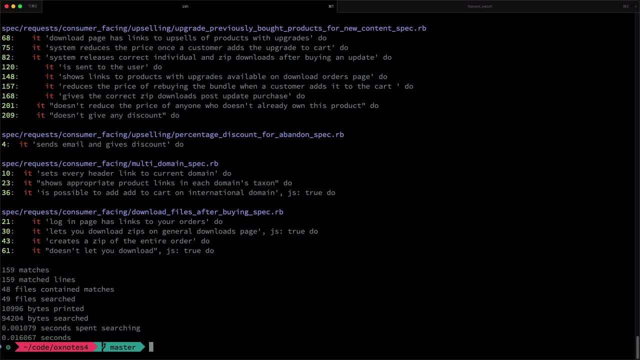 I have so much confidence in my code and I very rarely get surprise bugs in production for existing features. New stuff always has a few kinks to iron out. That's a given in software development, I think Basically this allows me to sleep at night Before I ever deploy to production. 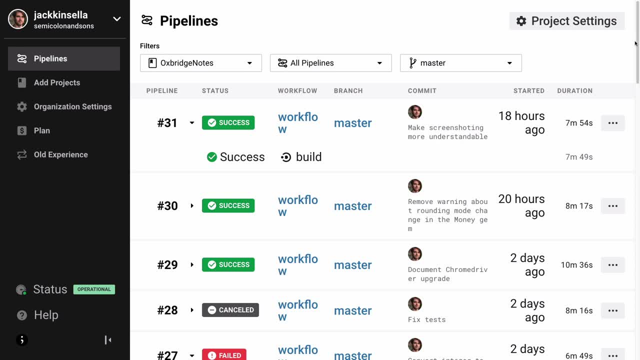 I run this entire suite of tests and ensure that they are passing. I do this on a continuous integration server because I don't want to slow down my machine. You can see here the tests succeeded for the last couple of commits and they failed here. I'm very happy that I detected this. 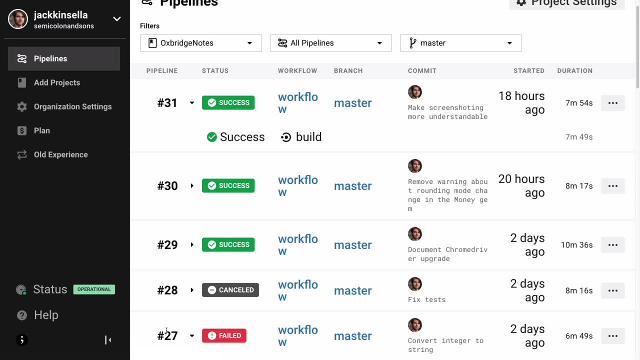 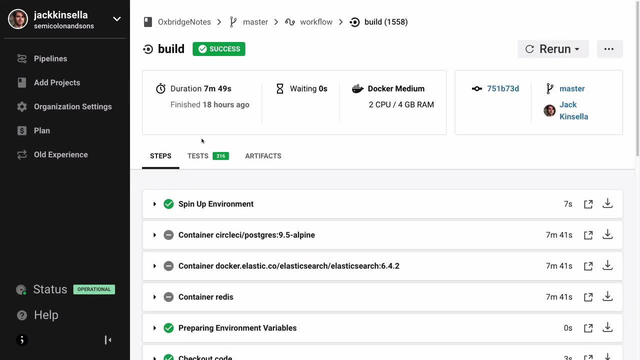 failure at the testing stage rather than in production, where the failures could have potentially caused havoc. These tests get run once for every commit. I pushed to GitHub. That way I never miss one. Let's look at how an individual test works First. you can see here: 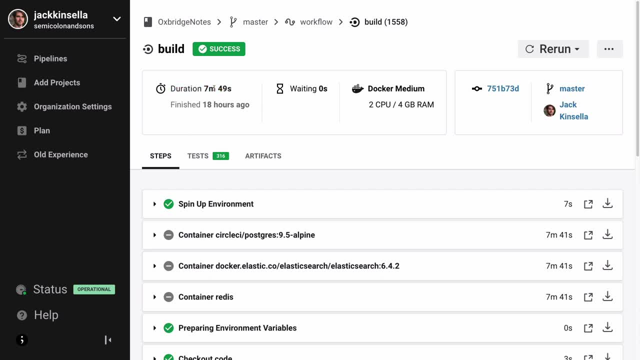 that the whole thing- building the environment and running the tests- took 7 minutes and 49 seconds. This is a region of 30 minutes when I had even less tests, but I've gotten better at writing fast tests in the interim. The tools have also improved. What basically happens here is we start. 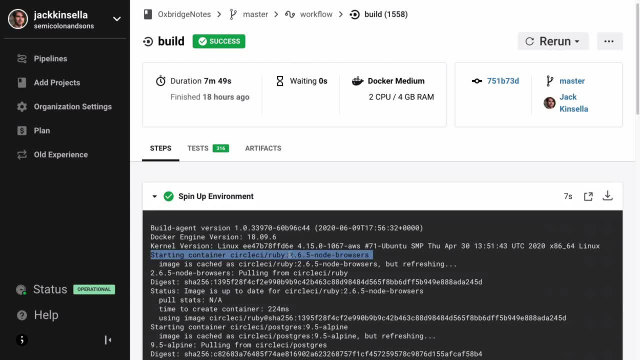 off by spinning up an environment. The important part here is that there's a CircleCI Ruby container with the particular Ruby version. I want Nodejs for running Webpack and the browsers for that sort of integration testing stuff. you saw especially the JavaScript stuff. Then I also. 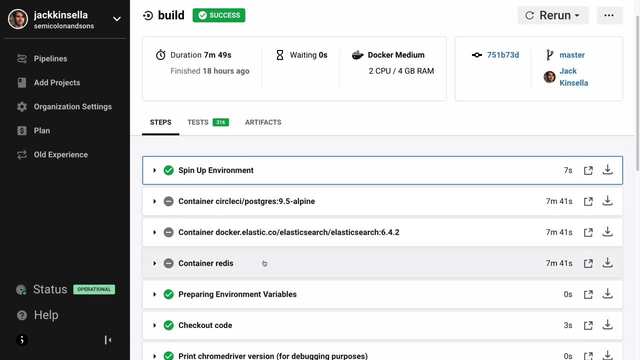 pull in my other major dependencies: Postgres, Elasticsearch and Redis. I use the real-life versions of these in my code to run the tests. I also pull in my other major dependencies: Postgres, Elasticsearch and Redis. I use the real-life versions of these in my code to run the tests. 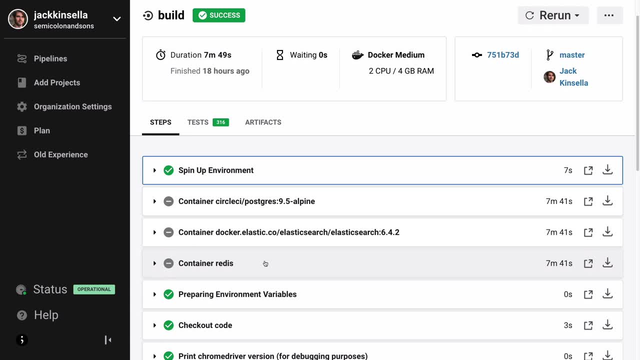 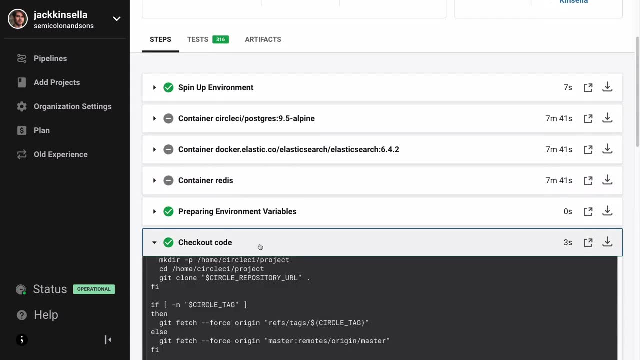 I use the real-life versions of these in my code to run the tests Because I want them to have parity with my actual production code. Some people would fake these things, but I think that's a bad practice for your integration tests. Next I check out the code. This, essentially, is pulling the code. 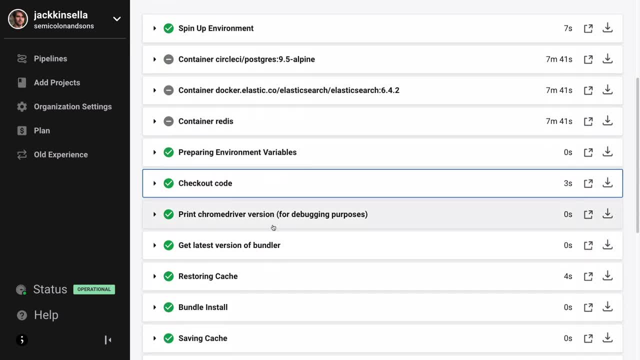 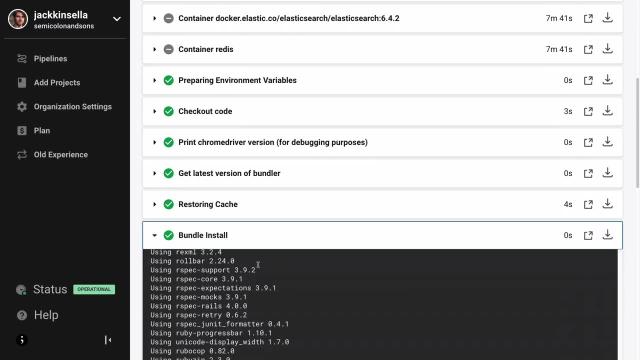 from GitHub into the testing container. There's some debugging stuff here. that's not important. The next important bit here is bundle: install. Bundle is the Ruby package manager. This is basically installing all my Ruby libraries I need. You'll have the equivalent in every other language. 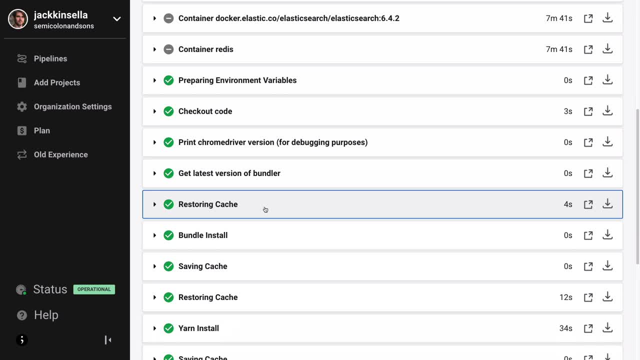 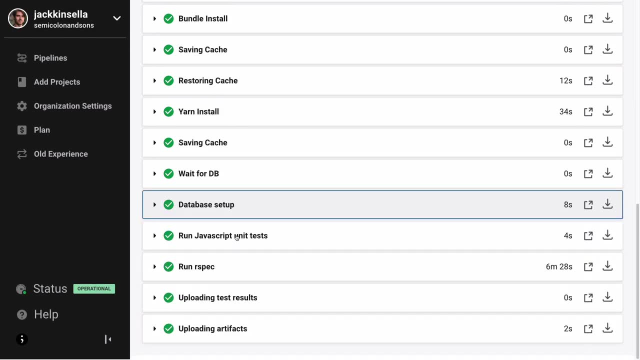 This can take a long time to download, so I cache these by taking a hash of the lock file. I do the same for installing and caching the JavaScript packages. Then I migrate my database, Then I start running the tests. There's a couple of JavaScript unit tests. That's not important here, The most. 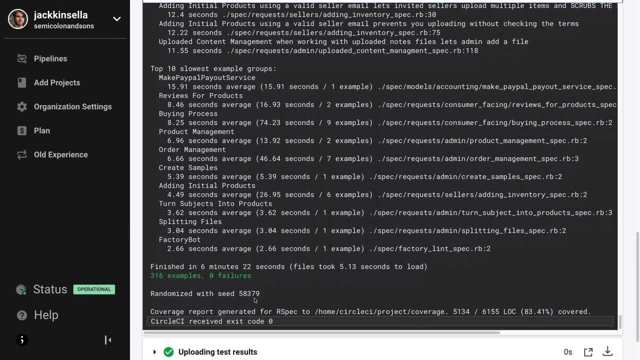 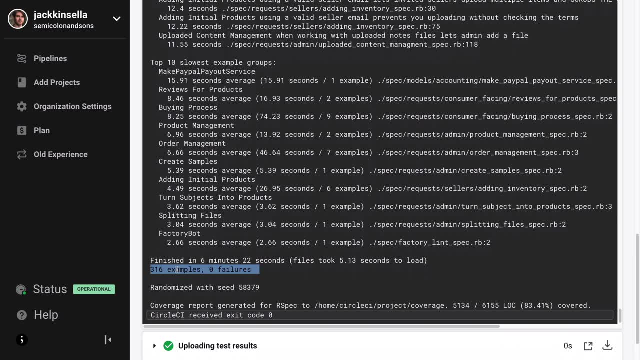 important bit is these RSpec tests. Here's the very bottom. You can see all the tests that got run. There's 316 examples. That is more than you would have seen previously, because I'm also including my unit tests here And you can see all these tests passed. That's very cool. For completion's sake, I 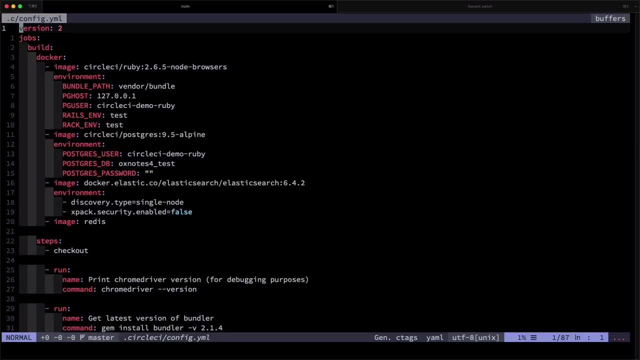 want to show you how I configure that continuous integration server. So I'm going to open up my CircleCI configuration server. I'm going to open up my CircleCI configuration server, I'm going to configyaml file And you can see here that I include this Docker image that you saw previously. 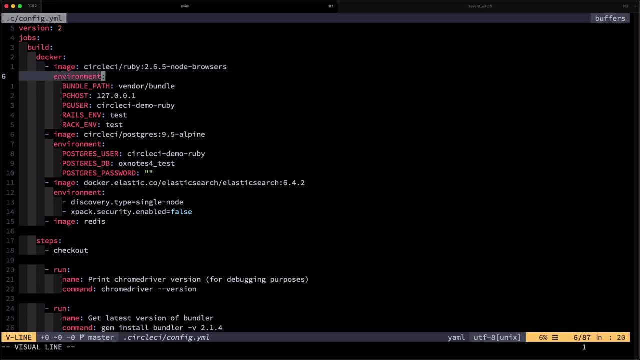 with Ruby and the Node browsers. Interestingly, here there are some environment variables. For example, I tell it where Postgres is and I tell it what environment to use in my Rails app- The test environment rather than the production environment, for example. Then I pull in the Postgres container. 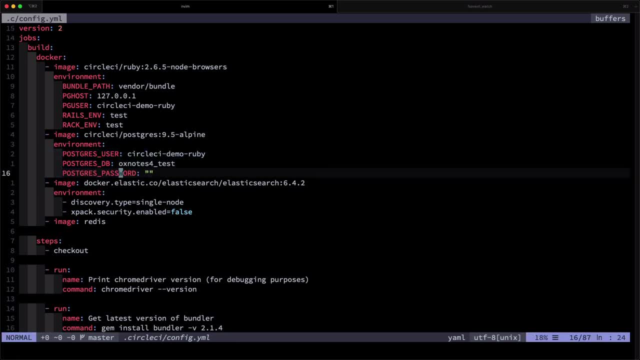 and set the Postgres user and database name and password. That has to be synced, of course, with my database configuration file in the Ruby land, As you can see it's done over here. Then I pull in my command to print my code And that's it. I need to see if I can do it, So I'm going to. 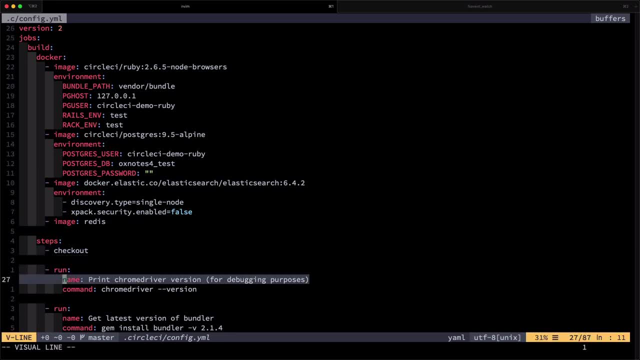 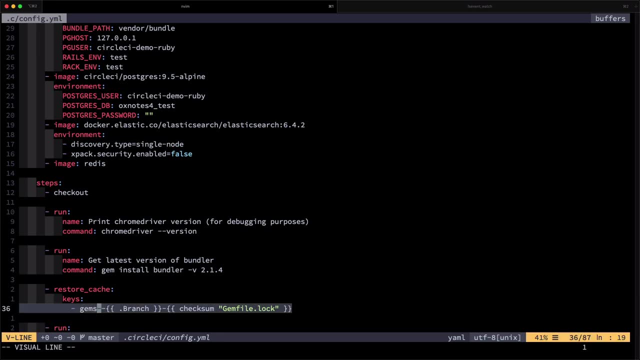 run a quick search and also redis. Next I check out the code. That's something built into CircleCI, I don't have to define that. Then I run a custom command to print the Chrome driver version. Then I install my package manager. Then this is to set up the cache with the checksum of my gem file lock. 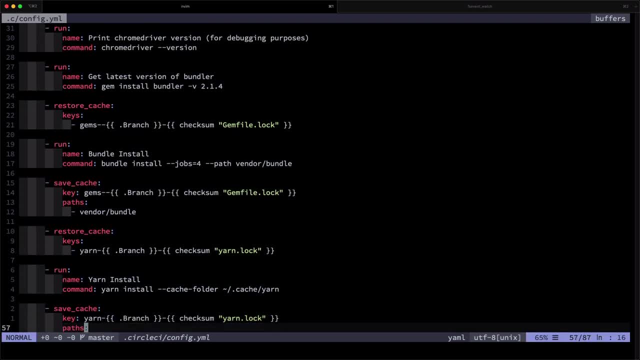 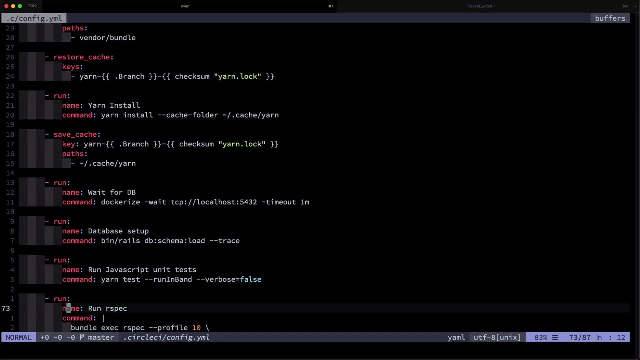 file, Then I install all my gems- if they've not been cached, Ditto for my JavaScript dependencies with Yang. Then I wait for the database to be ready, I migrate that database And then I start my Ruby or spec tests, And that's it. Creating that config file can be a lot of hassle. if you're 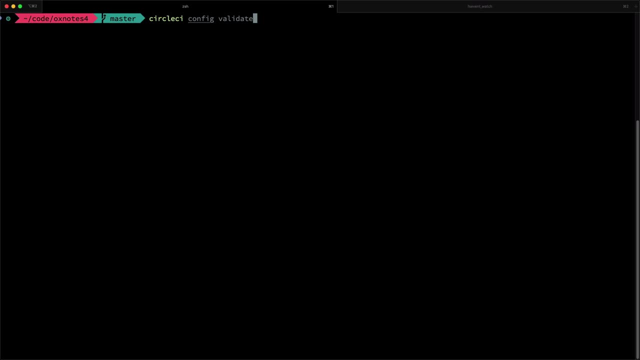 not familiar with the YAML file format- It's quite strict- Or with Docker And the development process would be very annoying if you were to constantly push to that remote continuous integration server to check if it was valid. But luckily you can validate that locally with this. 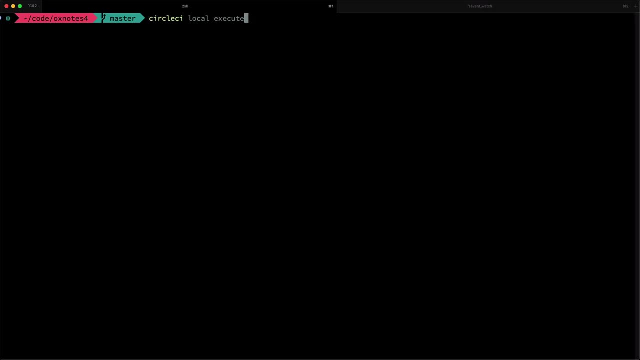 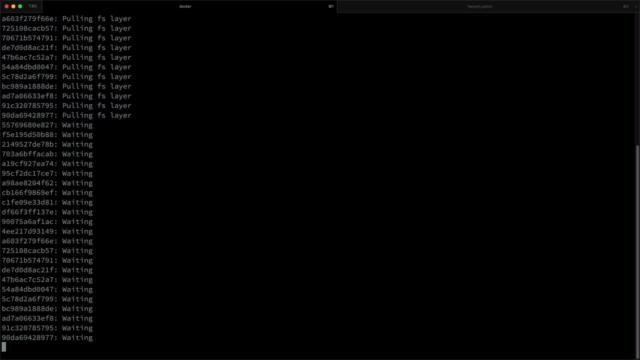 command to check that you haven't any syntax errors in there. A second tip is that you can also run all those tests locally on a localized Docker instance. This assumes that you have Docker already running on your machine. Be warned: this is often much more time consuming than the tests. 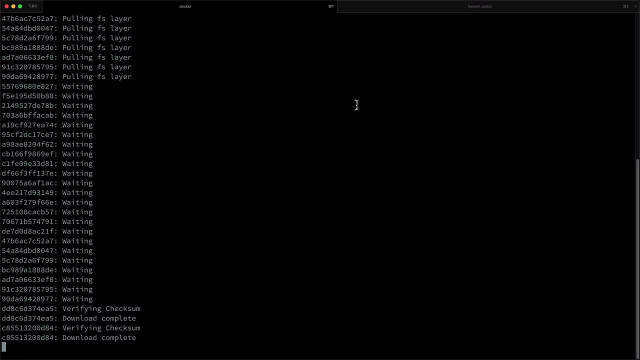 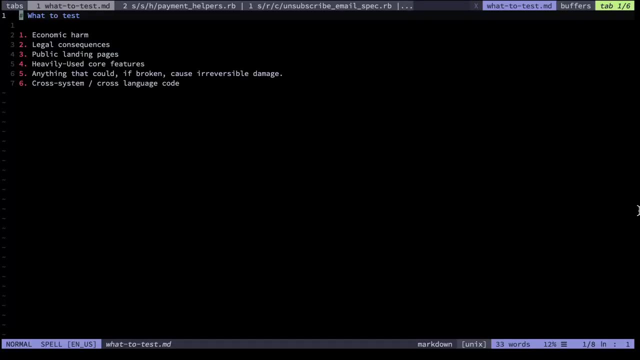 on the remote server. But the plus side is you don't have to make a ton of commits with messages like: try fixing CircleCI, attempt eight, attempt nine. Let me end this episode by talking about what to test Tests have costs. There is an initial upfront payment. in that you have to. 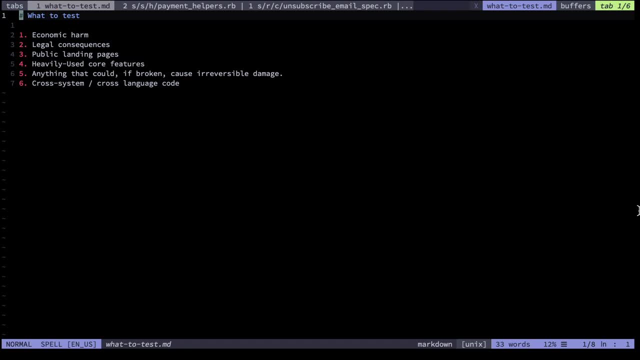 first write that test And then down the line. there's a bunch of maintenance costs. While more tests will lead to will usually lead to more robust code, the price you pay for that extra modicum of reliability may not be worth it in your case. I'm going to share my personal 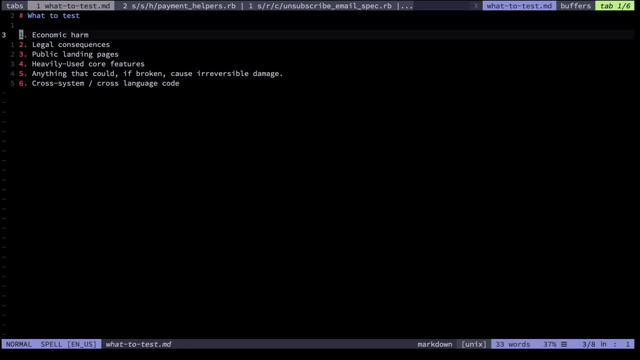 rule of thumb. here I'm going to share my personal rule of thumb. here I'm going to share my rules about what to test. The first is anything that's going to cause you economic harm. For example, I want to make sure that all my revenue generating flows keep working. I don't want to. 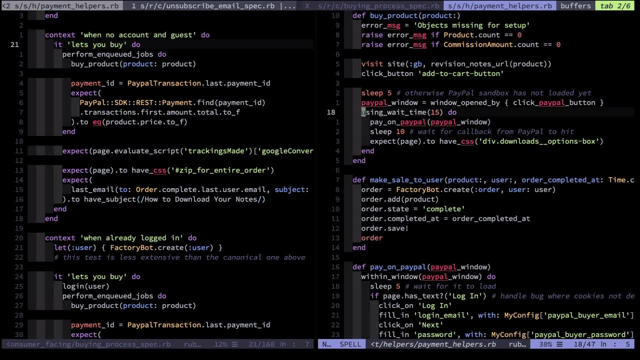 lose a day's worth of revenue. Most businesses don't either, And I do say that's a little bit controversial here. I literally test against the PayPal window that gets popped up. This is controversial in that I'm testing someone else's code- a third party vendor- But the advantage is. 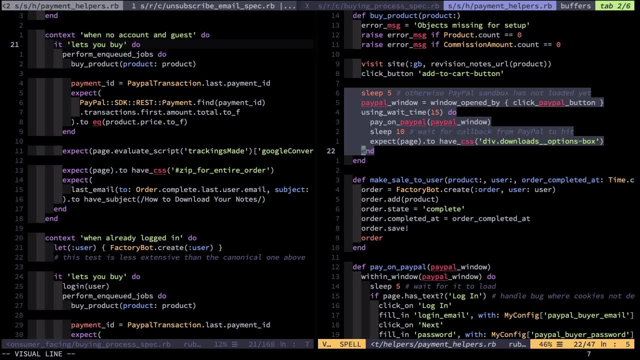 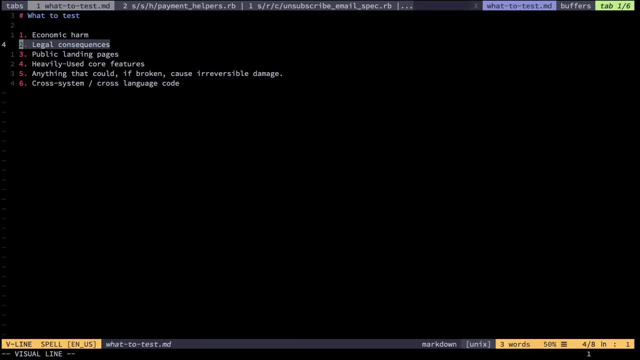 that I get to issue refunds against the sandbox PayPal API and transfer payments to sellers and all that kind of thing, And it gives me a hell of a lot of confidence that everything is working as it should. The next thing that's very important to test is anything that could have legal consequences, if you 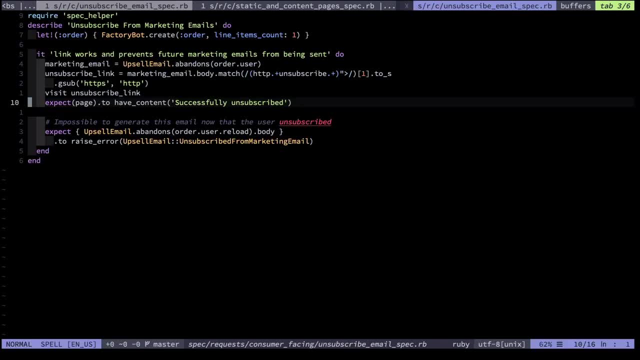 get wrong. In the case of most websites, you certainly want to be testing that your unsubscribed links work, lest you fall foul of the CanSpam Act. If you're a software vendor, you're going to want to make sure that your uptime is whatever you've promised in your contracts. And if you're selling, 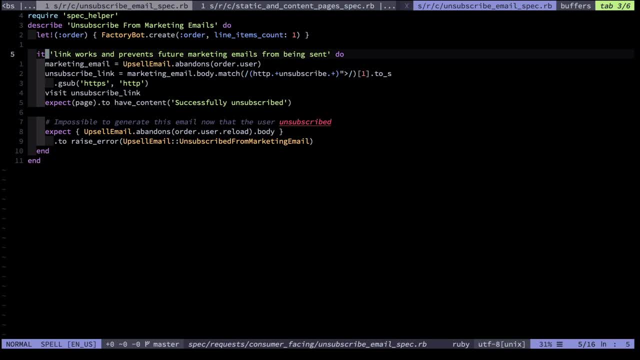 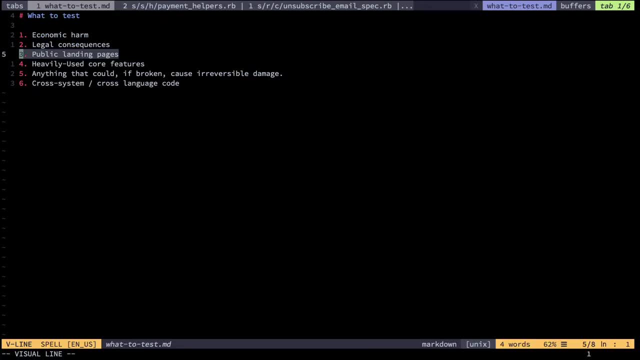 to consumers like I am. you're going to want to have to check that your VAT is calculated correctly, because you can do some serious jail time for mistakes in that department. The next important thing for me to test is public landing pages In the modern internet. 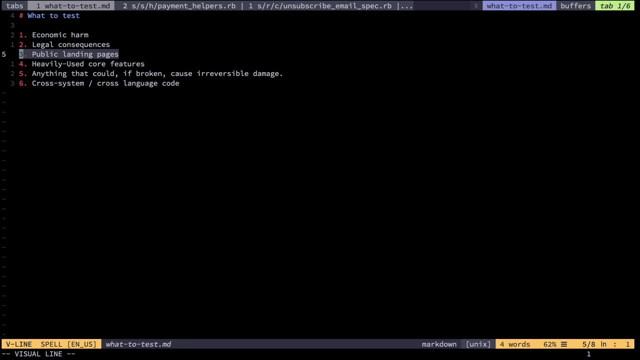 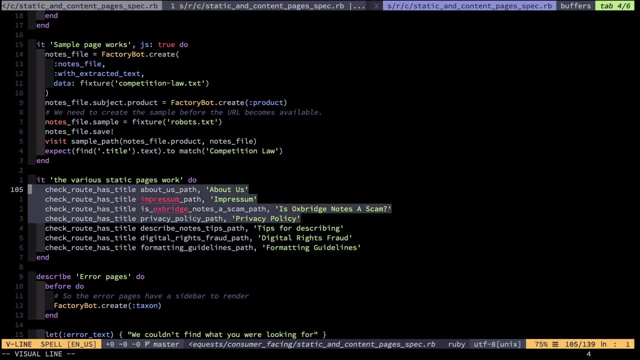 it costs a lot of money to acquire a user, to get them to your website for that very first time. It could be $30, it could be $100, it could be more. Therefore, you want to leave a very good first impression. In my case, I do things like check that my various static pages work, check. 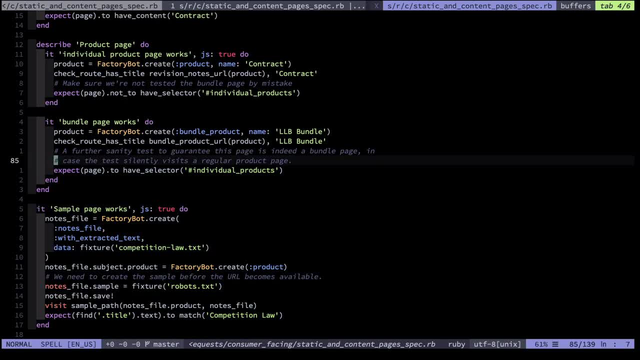 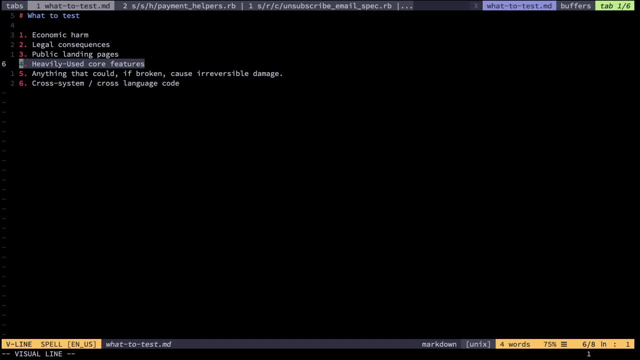 that all my kind of sample pages work, my product pages, that kind of thing. The next thing you want to test is any heavily used core features. This is basically an application of the 80-20 principle. For example, you want to check that your login continues working, all that sort of stuff. 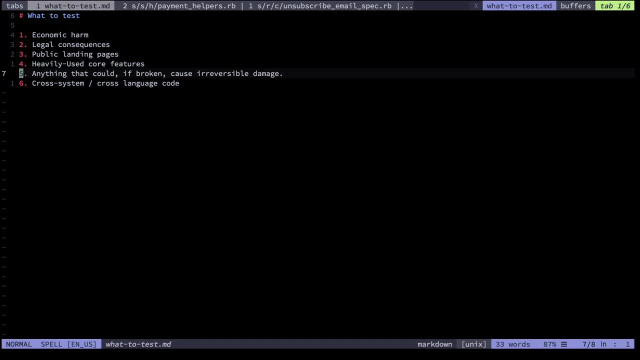 This is going to depend a lot on your particular use case. The next thing to test is anything that, if broken, you're not going to be able to use. If you're not going to be able to use it, you're not going to be able to use it. If you're not going to be able to use it, you're not going to be able to use it. 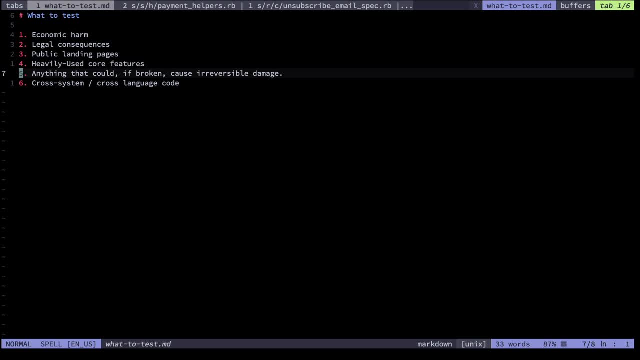 If you're not going to be able to use it. you're not going to be able to use it- Could cause irreversible damage to your business. This won't necessarily be a browser test, but it also might be In the case of my code. I could tell you one thing: that could cause irreversible damage for sure. 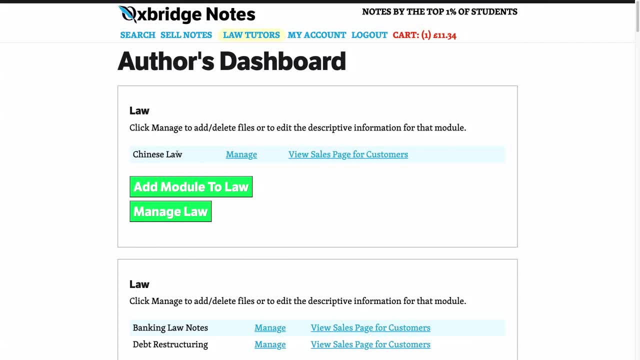 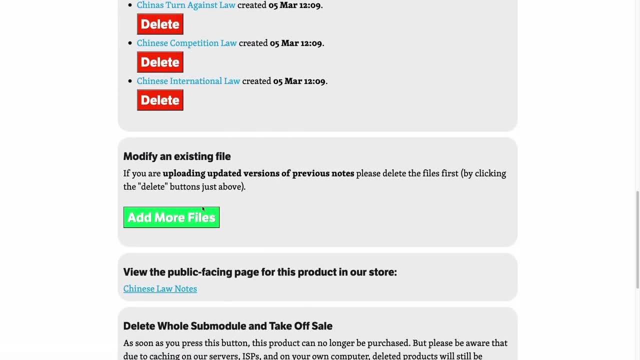 I'm going to give you an example here. Authors upload these subjects that they sell on my website. For example, here's Chinese law on sale. Let's go into the management page here. You can see that there are a bunch of files which the author uploads, and they can add more files here. 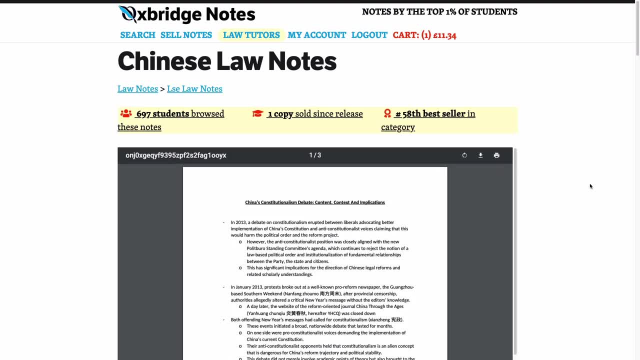 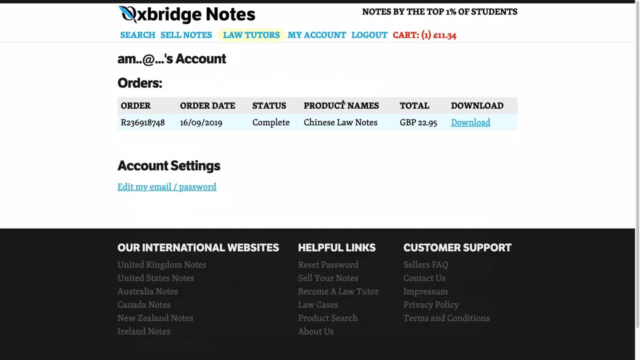 This is the corresponding product on sale in the front end. Random customers will buy that. Now I also allow sellers on the website to delete any product they've uploaded. But you can see a problem here. What if some customer like this one here has already bought? 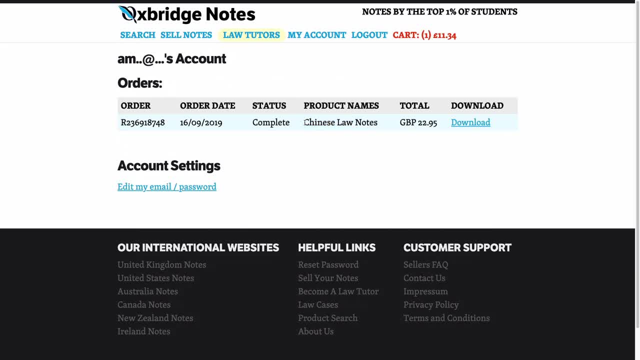 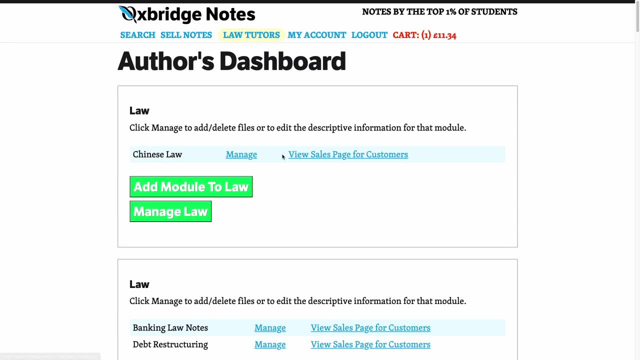 those Chinese law notes, but the seller has deleted it ever since. I still need to honor that contract to the purchaser of those notes. Therefore, I can delete everything that that seller has uploaded- If you look here, all these other subjects that they have, but I can't delete. 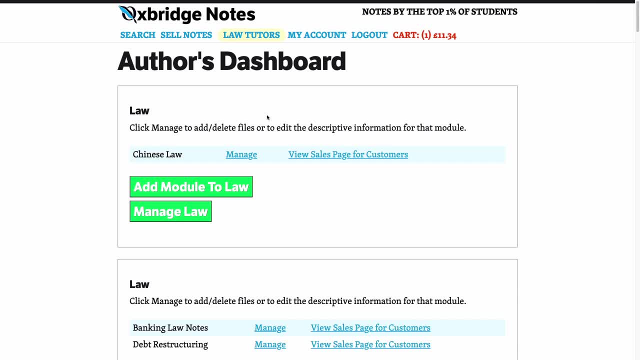 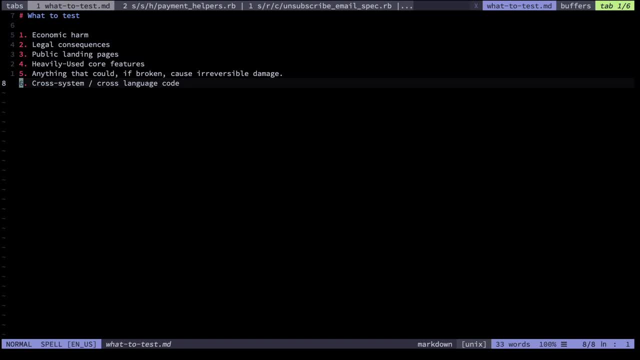 that Chinese law. I have to keep that present in order to be able to honor those downloads. Therefore, I test against this particular error case within my code. The final thing I find important to test is whenever there are systems that go across language barriers.